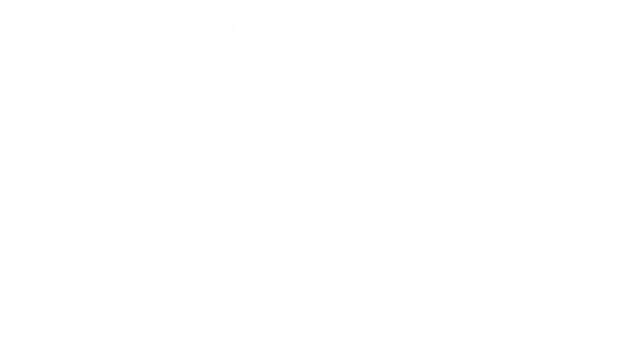 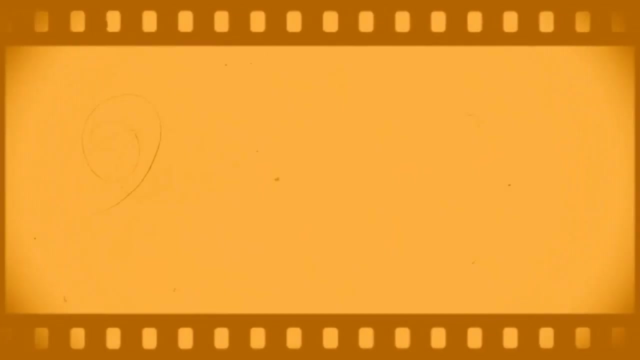 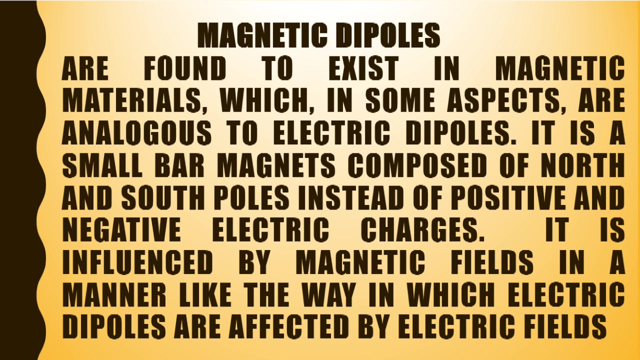 Answer: magnetic material Present in countless tools of modern life. these materials, because of their importance and complexity, make research on magnetism intense nowadays. Why do we have to study the magnetic properties of a material? One of the familiar examples is a compass. 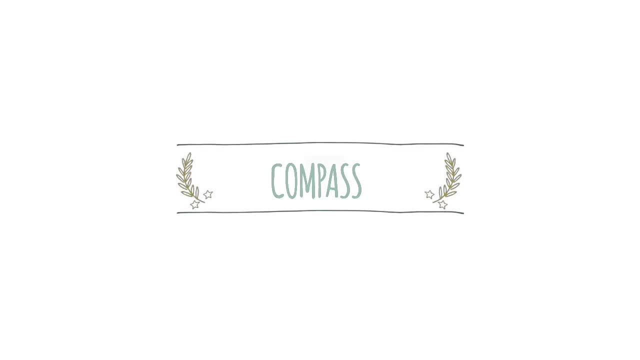 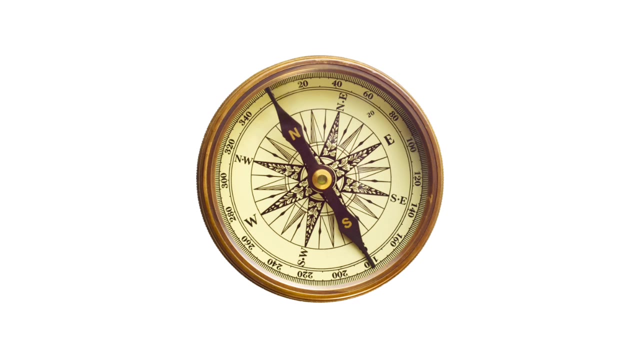 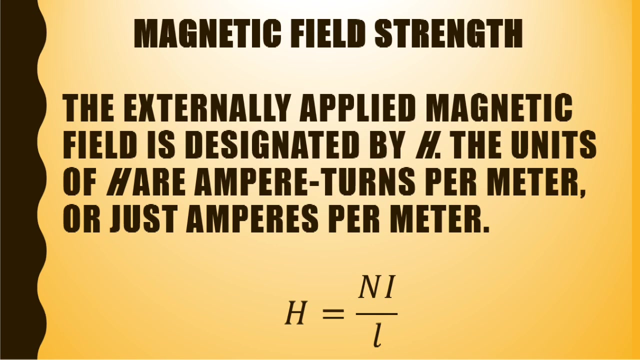 Why do we have to study the magnetic properties of a material? It makes a magnetic compass little and supra-directs a magnetic field that is used for navigation. Why do we have to study the magnetic properties of a material? Answer: magnetic material. 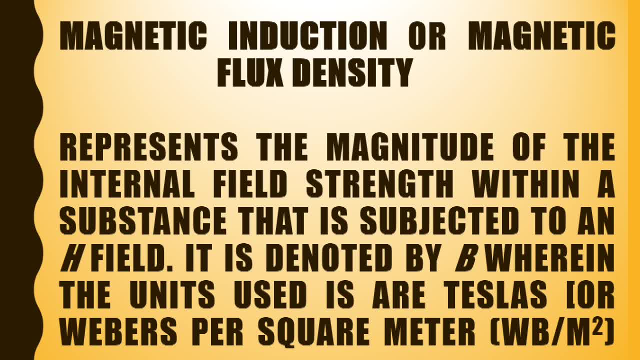 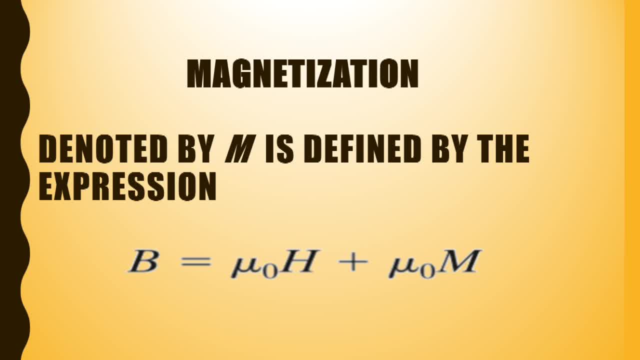 Why do we have to study the magnetic property of a brain that is used for magnetism? The answer is: Does it give me the time to study? No, it's not possible. The answer is: if it gives you the signal to sit in magnetic position, whether you are wearing glasses or wearing a mask. 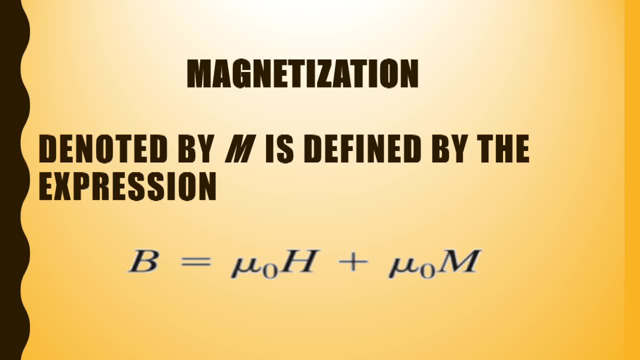 simplesmente. the센user shaft is the ring. no matter how high or high you are in the space, then the second minute you fall flat on the surface, you will definitely take the second minute, And if you fall to the left half you will fail the second minute. 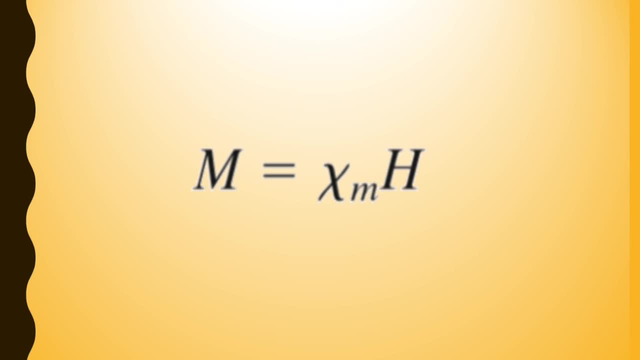 and the third minute you fall to the left half of yourATHBOTY script and lose the third minute. you cultivate Ultimately magnetism fifty degrees down. That's all I can say. mulher maki n manuscript nas Richard ren branches a파 arrangement mega kasl. 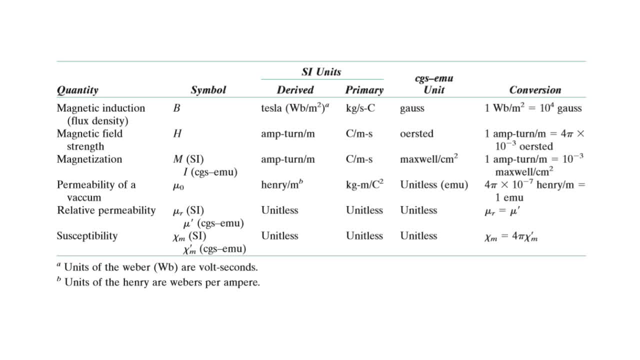 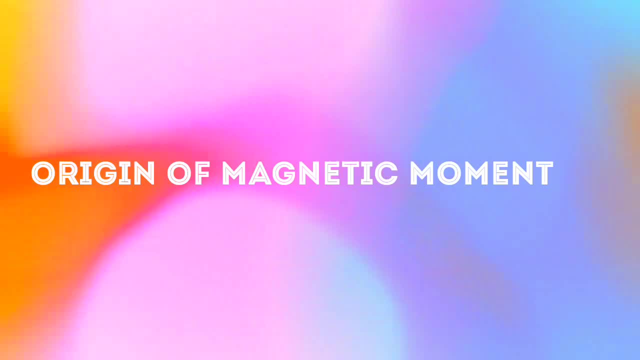 but for marriage. the iagain revelation, nika from online Magnetic units may be a source of confusion because there are two systems in common use. The units for both systems, as well as the appropriate conversion factor, are contained in this table. The macroscopic magnetic properties of materials are a consequence of magnetic moments associated. 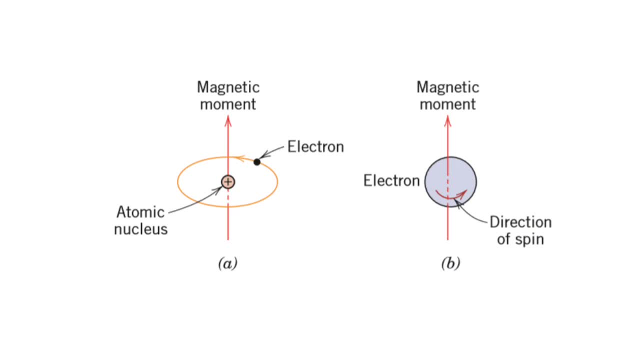 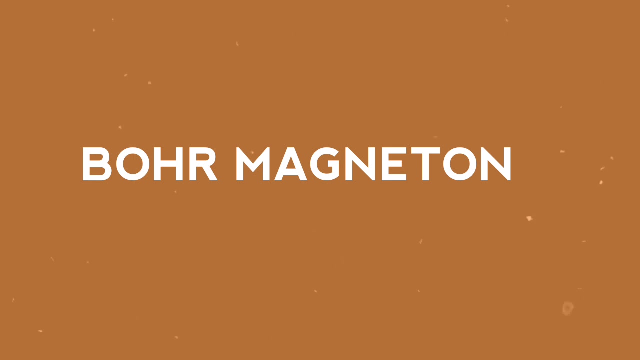 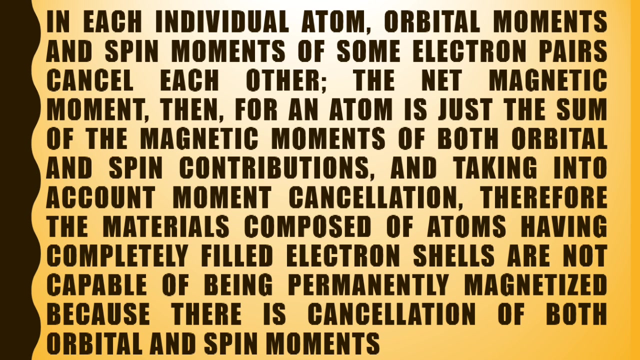 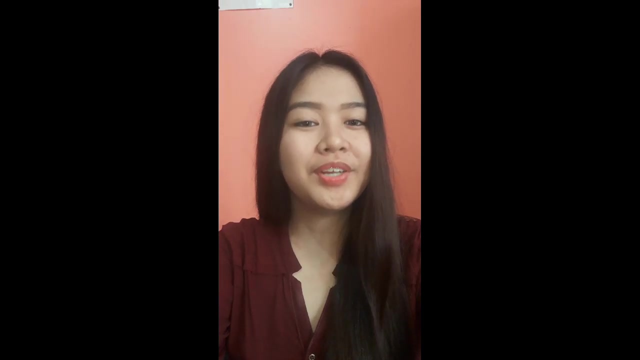 with individual electrons. In this diagram. each electron in an atom has a magnetic moment that originate from two sources: an orbiting electron and a spinning electron. Bore magneton is the most fundamental magnetic moment. There are three types of magnetism: diamagnetism, paramagnetism and ferromagnetism. 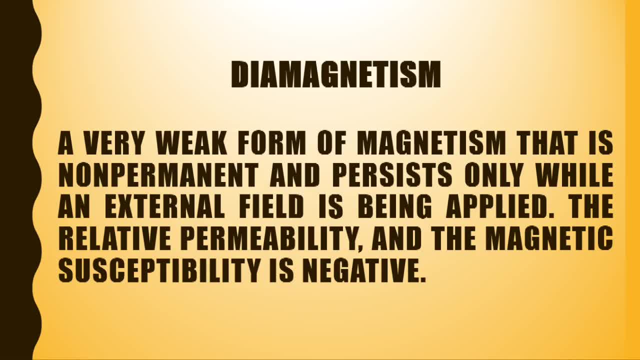 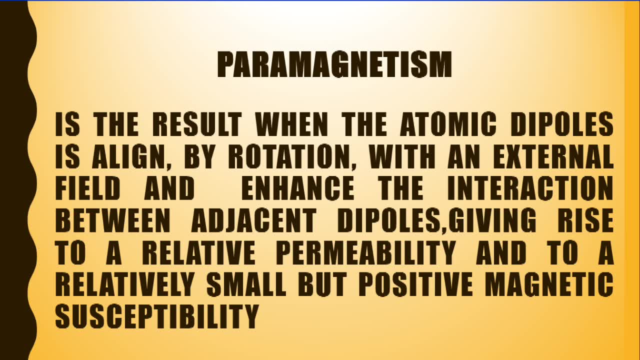 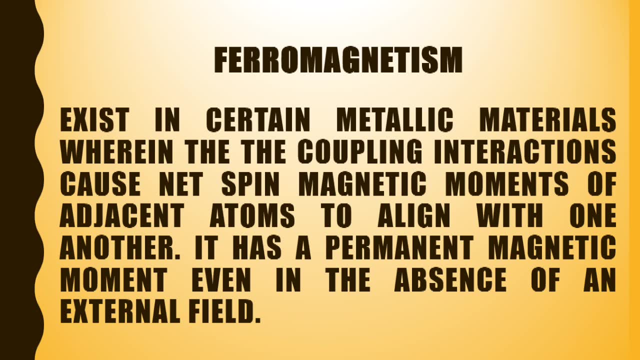 It is found in all materials, but because it is so weak, it can be observed only when other types of magnetism are totally absent. It is displayed in the transition metals like iron, cobalt, nickel and some of the rare earth metals such as gadolinium. 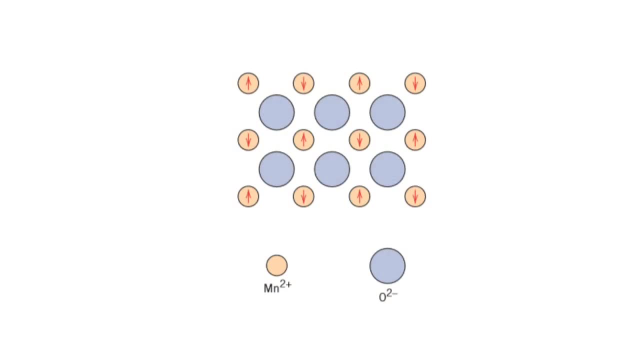 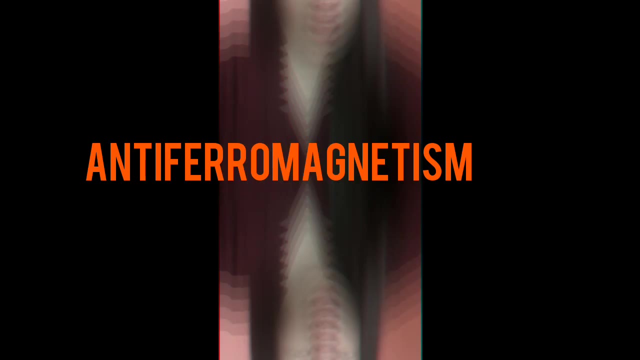 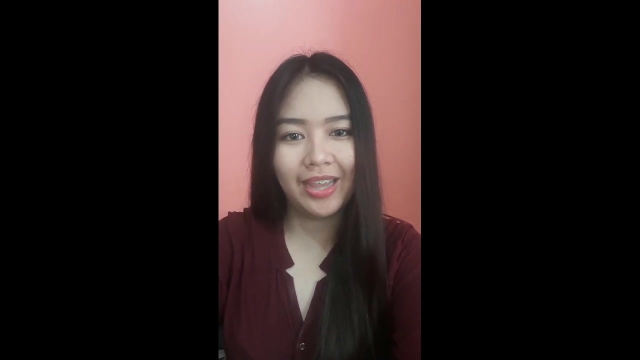 In this diagram we could see the antiparallel placement of spin magnetic moments in the manganese oxide. This phenomenon is called antiferromagnetism. The phenomena where in the material exhibit a permanent magnetization is called ferromagnetism. Cubic ferrites, hexagonal ferrites and garnets are ceramic materials that are ferromagnetic. 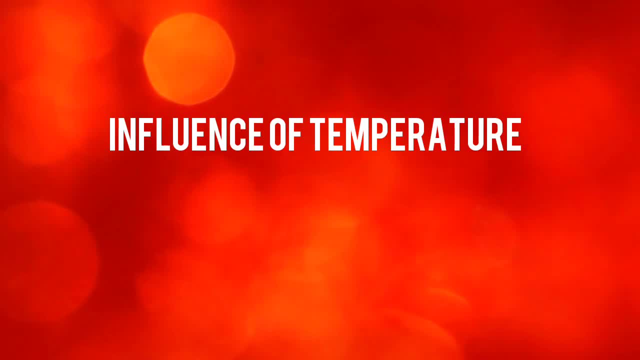 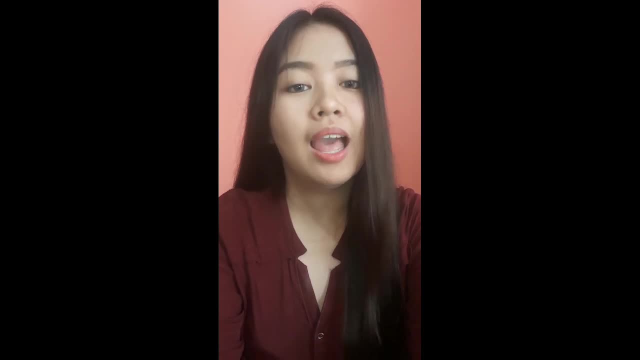 For ferromagnetic antiferromagnetism is a phenomenon where the ferromagnetism of a ferromagnetic material is observed in the material and the ferromagnetism of the material is observed in the material. In the case of ferromagnetic, antiferromagnetic and ferromagnetic materials, the atomic thermal 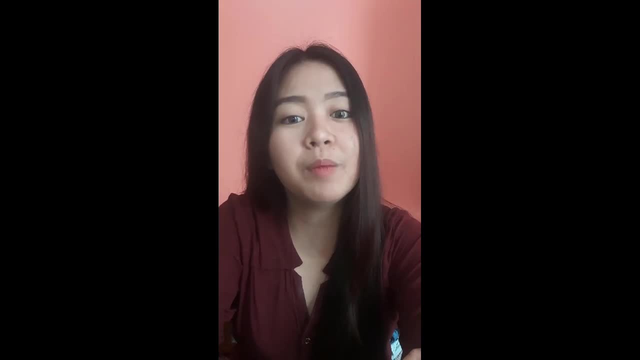 motion counteracts the coupling forces between the atomic dipole moments, causing some dipole misalignment, regardless whether there is an external field present. With increasing temperature, the saturation magnetization diminishes gradually and then abruptly drop to zero at what is called the current temperature. 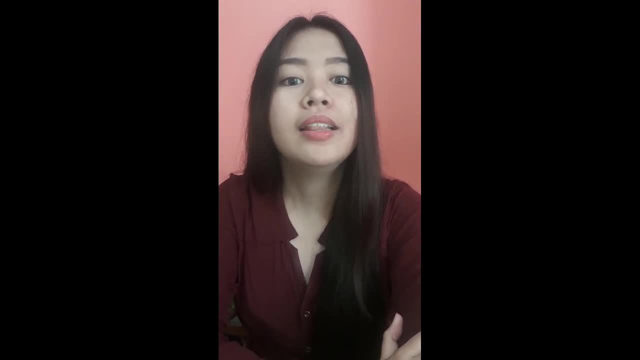 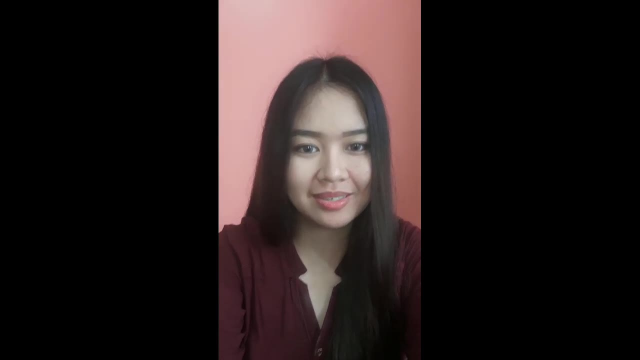 Where in the antiferromagnetic material that have temperature above this point becomes paramagnetic. Now let's talk about domain and hysteresis. Hysteresis, behavior and permanent magnetization may be explained by the motion of the domain walls. But first let's define domain. Any ferromagnetic or ferromagnetic material that is at a temperature below current temperature is composed of small volume, region in which there is a mutual alignment between the two zones. The domestic dipole moments are still aligned in the same direction. in the same direction. 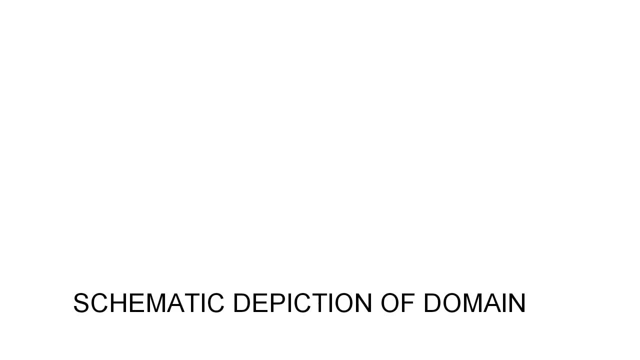 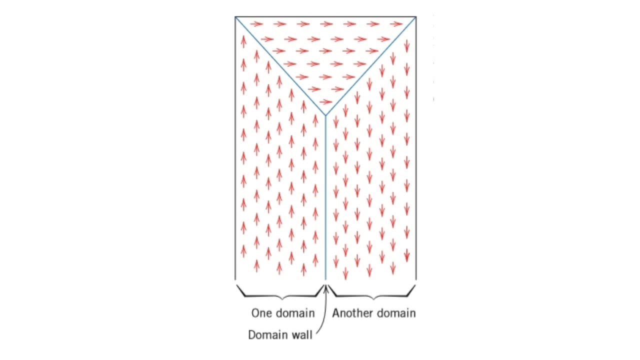 for all magnetic dipole moments. This is what we call the domain. the domain. The domain arrow represents atomic magnetic dipoles. Within each domain, all dipoles are aligned, Whereas the direction of alignment varies from one domain to another. 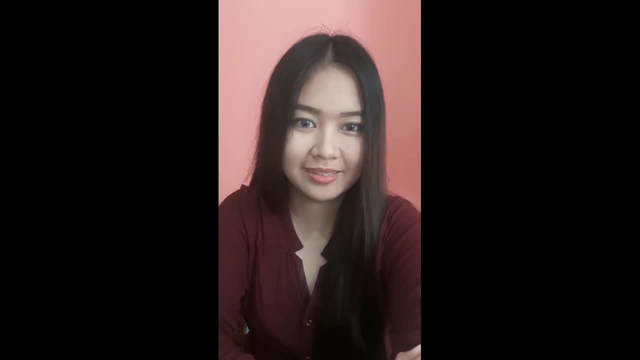 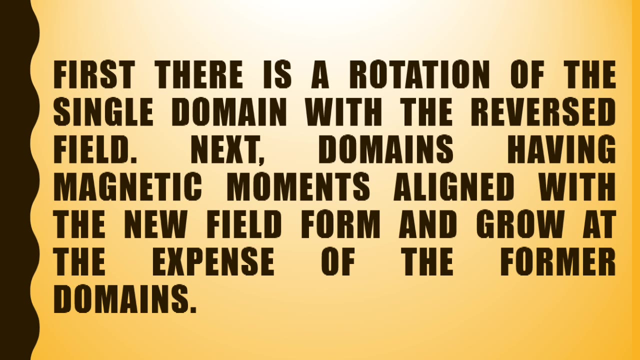 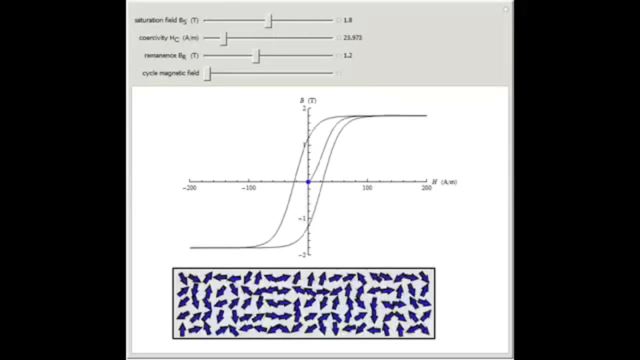 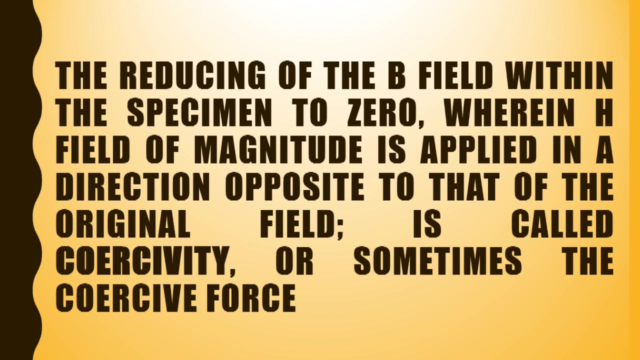 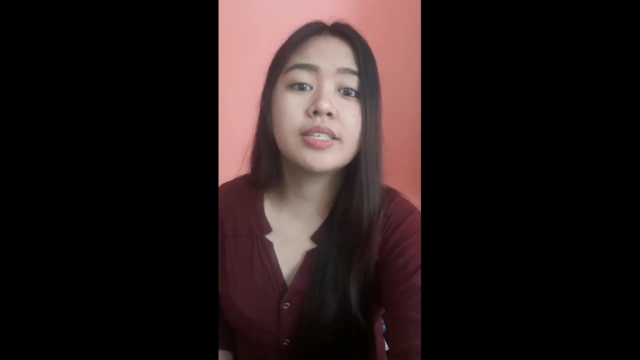 Now, how does hysteresis happen? The resistance to movement of domain walls that occurs in response to the increase of the magnetic field in the opposite direction accounts for the log of B with H or hysteresis. Both ferromagnetic and ferromagnetic materials are classified as either as soft or hard on. 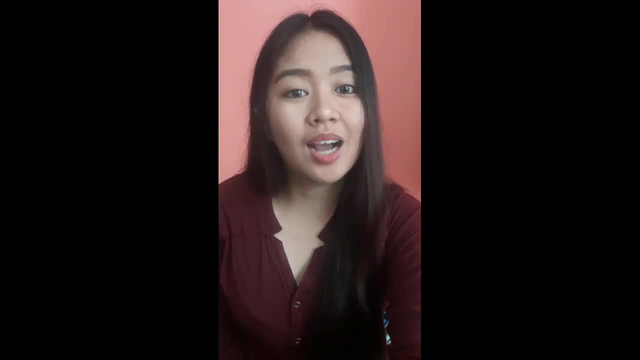 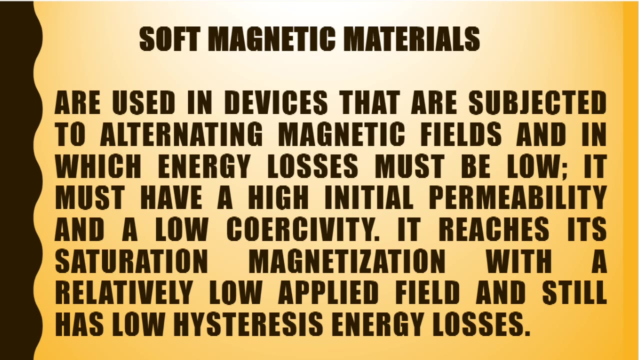 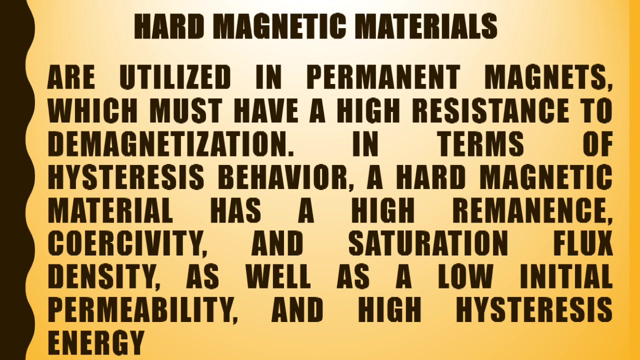 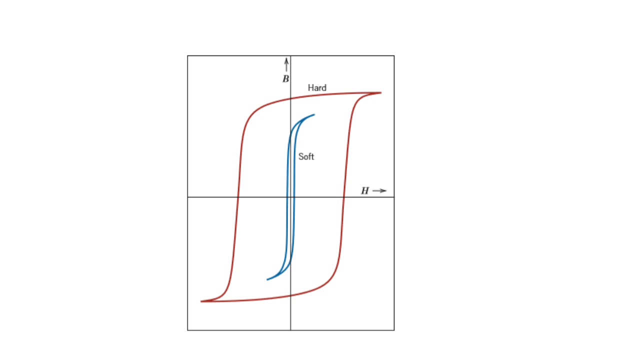 the basis of their hysteresis characteristic. So let's discuss the difference between these two. Alloys composed of irons are soft magnetic materials that are used in generators, transformers, motors, dynamos and switching circuits. This is a schematic diagram for soft and hard magnetic materials. 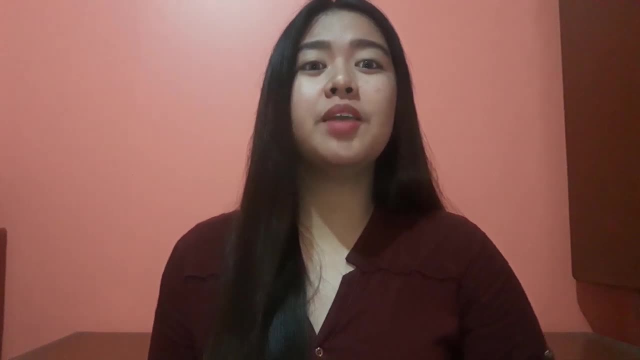 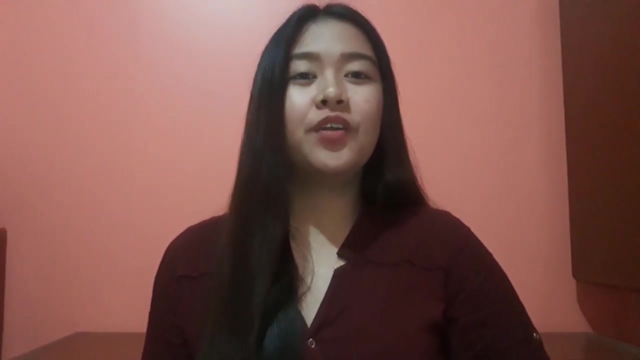 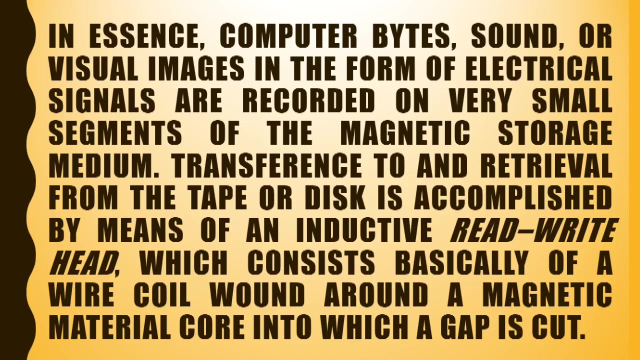 Within the past few years, magnetic materials have been used in various forms. These materials have become increasingly important in the area of information storage. In fact, magnetic recording has become virtually the universal technology for the storage of electronic information. When the gap is cut, data are introduced by the electrical signal that generates magnetic. 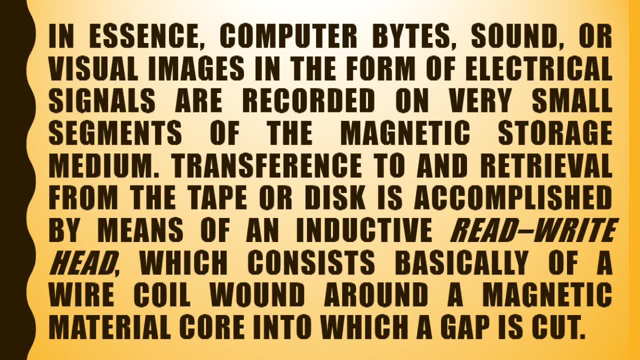 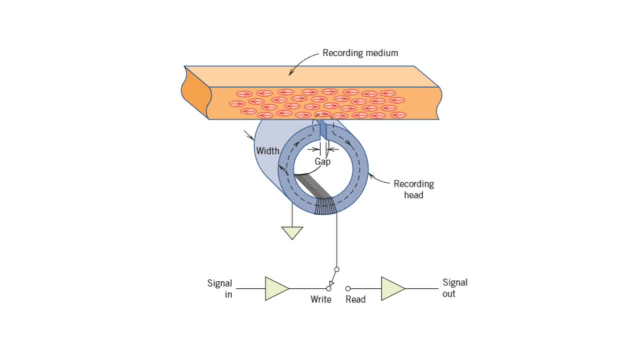 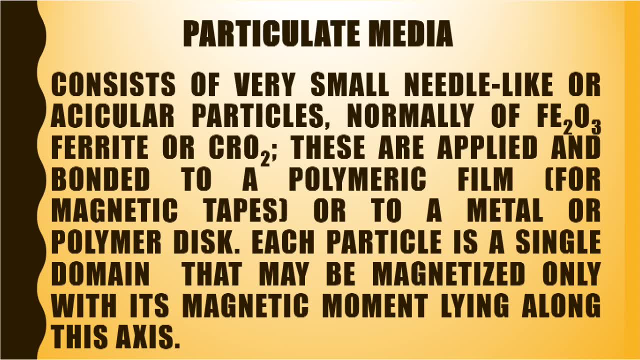 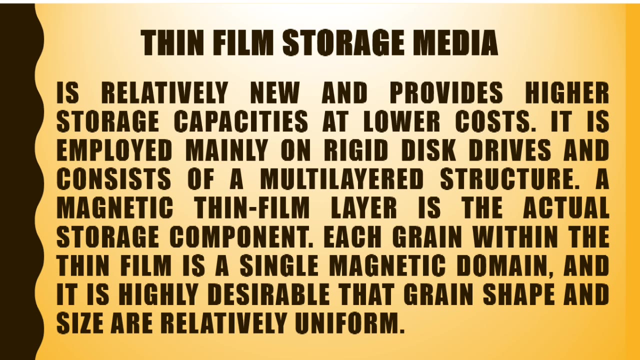 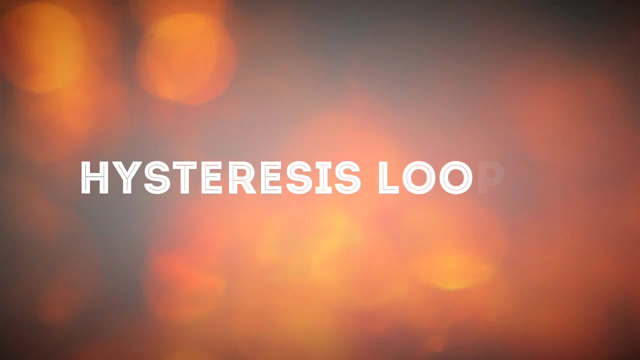 field that magnetizes small area of the disk within the proximity of the head. This picture shows how information is stored and retrieved using a magnetic storage medium. Historicist Loup's for this. magnetic storage media should be relative large and square. Historicist's loops for magnetic media- Strolitz medium should be relatively large and square. 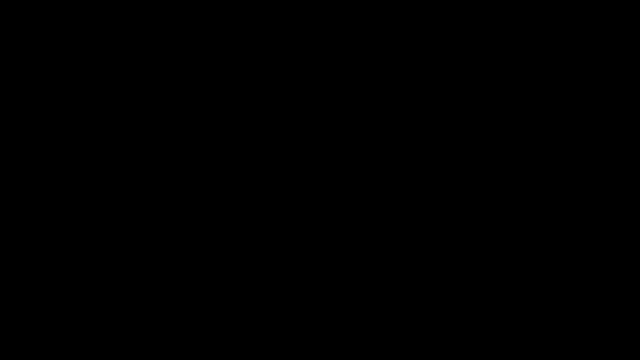 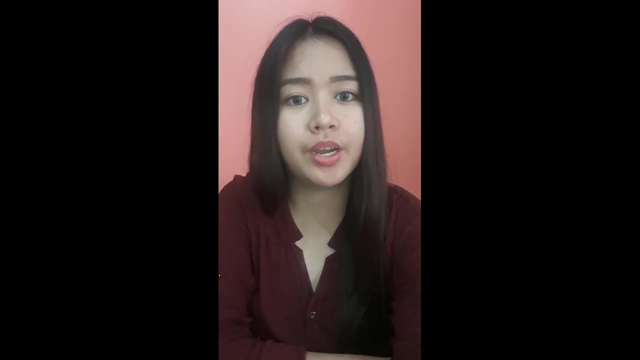 characteristics ensure that storage will be permanent. There are materials that displays a behavior in which resistivity at a very low temperature abruptly plunges from a finite value to one that is virtually zero and remains there upon further cooling. These materials are called superconductors.